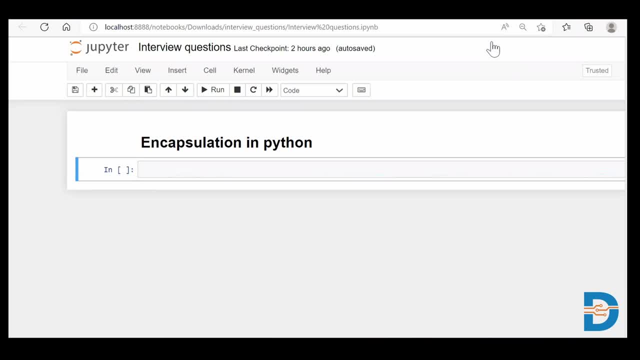 nothing but a concept on which, you know, we just encapsulate, which means that you know there is a capsule and in that capsule we put all the data, all the methods, all the variables and just close it up. So basically, if you talk about a class itself, let's say: 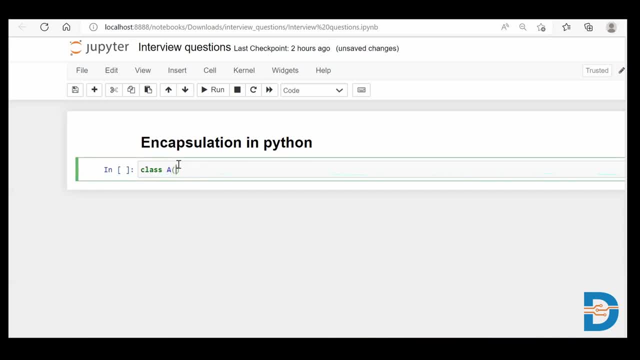 I am defining a class. let's say I'm defining a class. let's say A: okay, And inside of this class, I'm going to, you know, create one variable, call it to be var and simply I'll just name it. I am a. 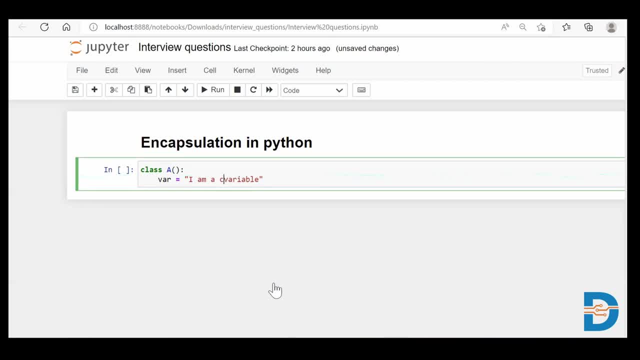 Very able, right Class variable And I'll just create one constructor for it. I'll say to be. let's say, let's say one functional, create not a constructor. Let's say I'm creating one function, Print. So work of this function is to just to print. hello, that's it. So 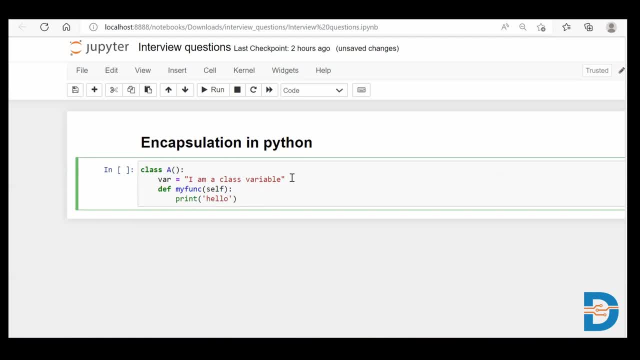 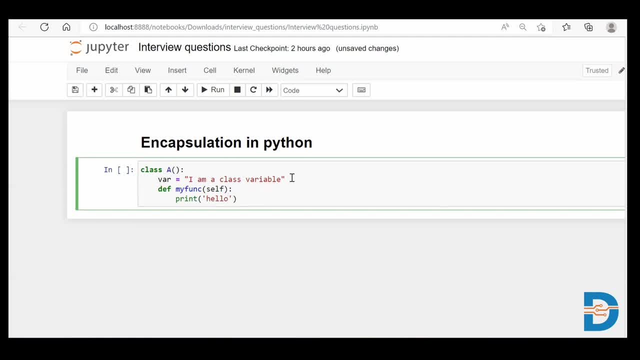 means take a piece of block and write all the variables and all the functions within that particular block, such that the scope of that variable and function is limited inside that class itself. So right now, what I have done? I have just created one class Inside. 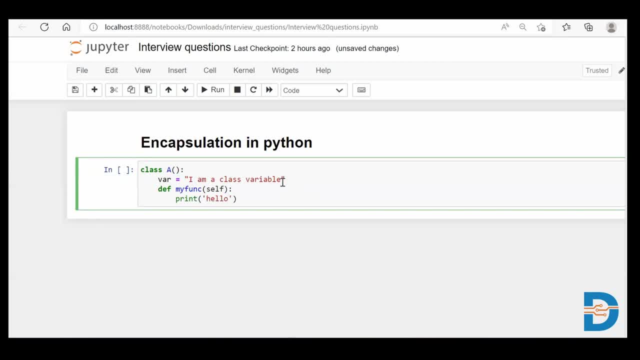 that class, I have just created one of the variable and inside that class itself, I have just created one function. right now, if i run this, right now, if i create an object of this class, okay, like this: so this is an object. and now, if i want to, 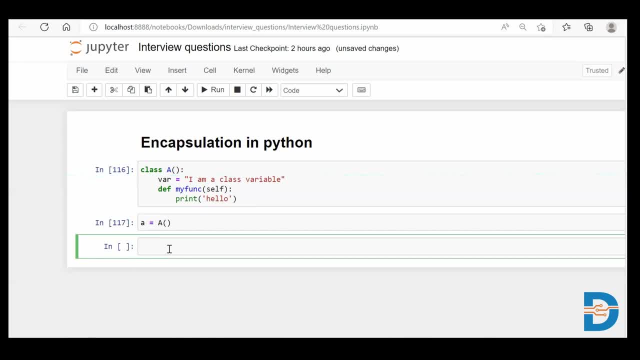 retrieve back the variable that i have created inside the class, i can use a dot back. so this is an attribute and you know not an attribute. basically, it's a variable, class variable, and if i want to call the function which has been made inside the class as well, i can simply write. 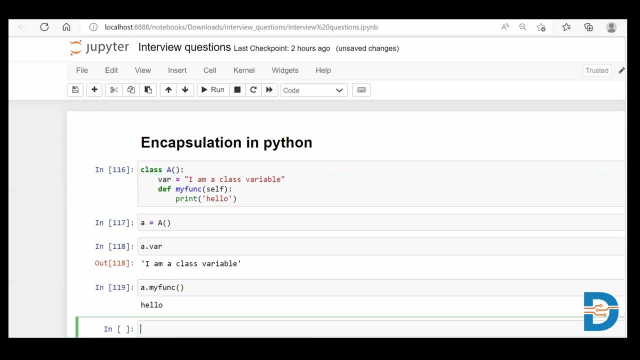 a dot my punk and it will give me back hello, uh, the thing is, this is a class and all the variable and the function that we have created it has. a class are the public classes. and public variable means is its scope is not just limited inside this class itself, but outside the class. 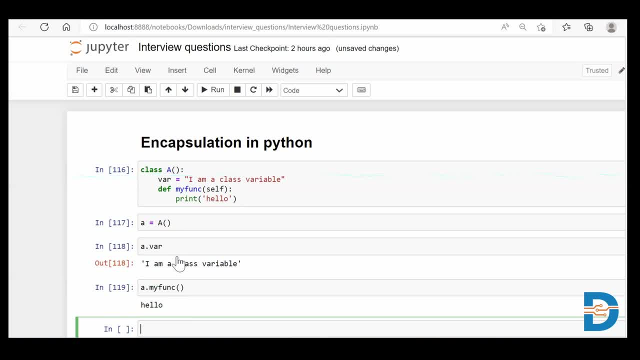 also these functions and method can be called in order to restrict these things. i require to make this variable and these functions as a private and or in order to make it private, all i require is to make double underscore, starting with double underscore and the name of the variable. so, 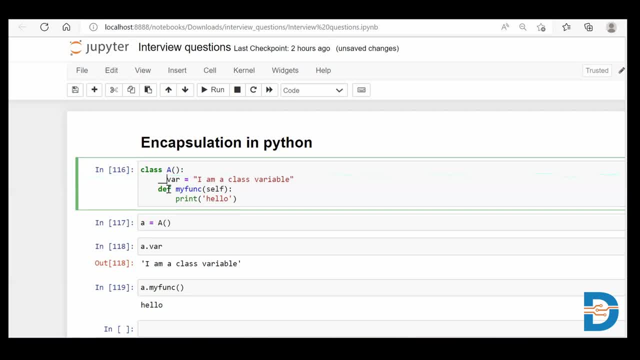 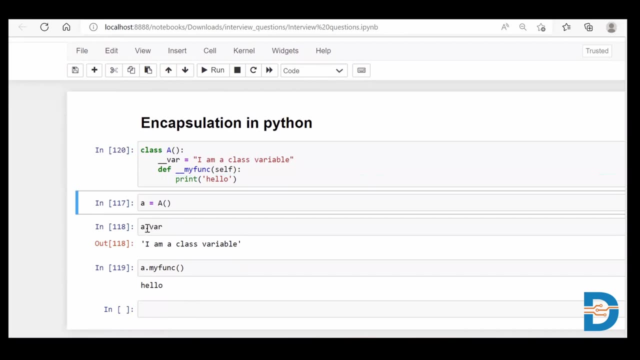 the variable that i have defined has now become a private variable, and so does. if i want, i can simply use double underscore for the function as well, and this function has now become private as well. so now, if i run this, now if i simply try to call this, let's say, double underscore var, like that, and 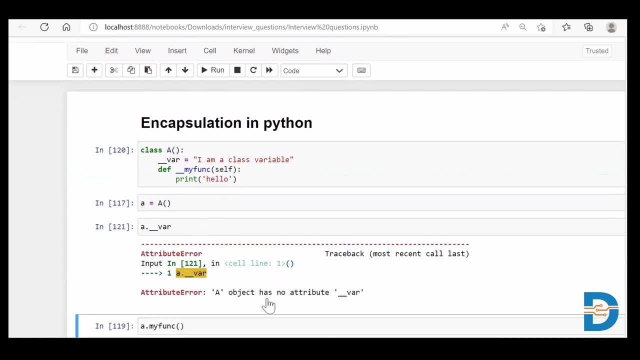 i simply run this, i'll get an error saying that a object has no attribute: underscore, underscore var. now over here you can see that i have done underscore- underscore- var, but when i'm calling this variable outside this class itself, it's showing me error saying that underscore, underscore. 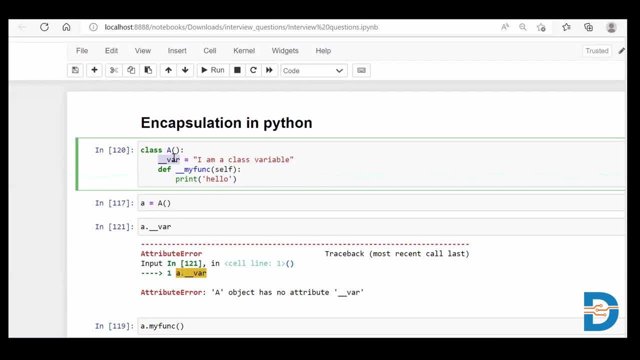 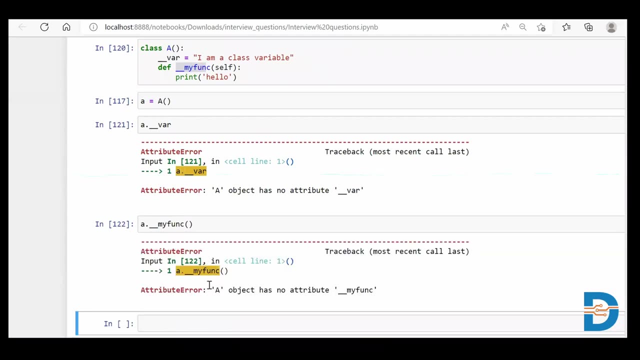 var is not defined. the reason is this variable is a private variable now, so it can be only used inside the scope of this function. and if you see this function itself, this function is also now. if i call my function- let's say i call my function like this- it will say that a object has no attribute. i mean, it is not understanding. 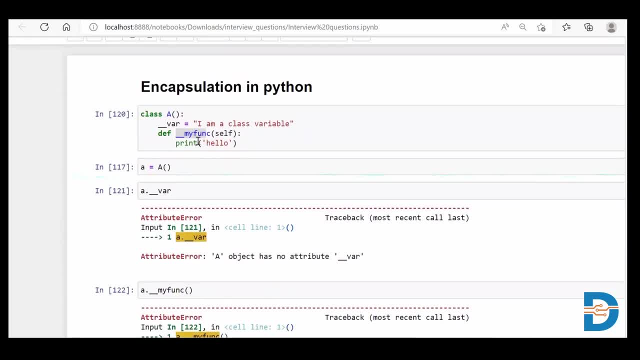 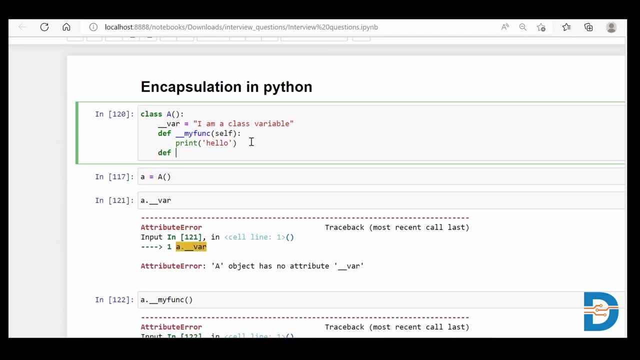 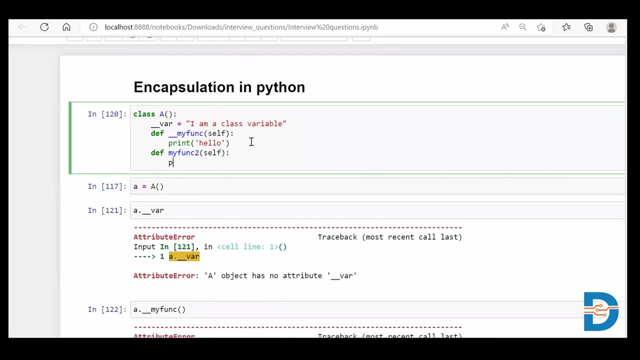 what exactly is happening with you know these kind of things that you are trying to call, because actually that's a private one. so if i simply use one function, let's say def my func two, i found two, simply self. and now if i use again the print statement saying that, 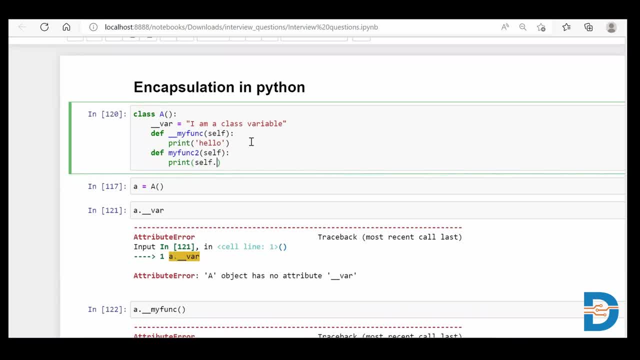 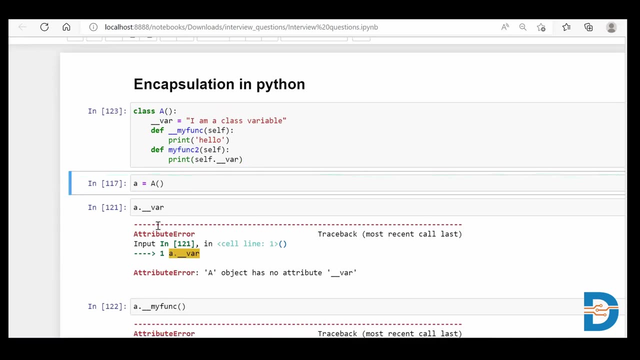 uh, what i said, simply use self dot underscore, underscore var. so what is happening? that inside this function only i am using this variable underscore underscore var, and this has been defined in our function, my func2. now, if i run this and now if i let me just put one more black, some more self dot underscore var. 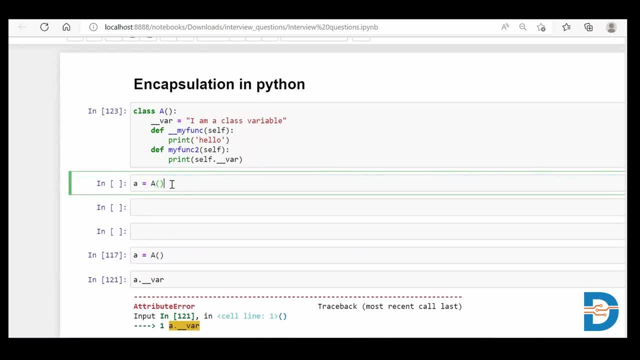 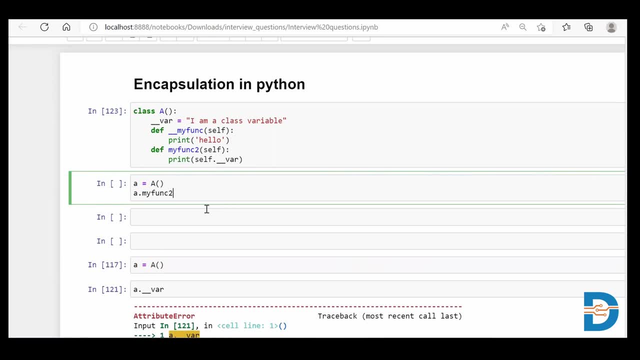 over here and now, if I simply a equals to a means, I'm creating the object of a. and now if I say a dot, my func two means what I'm doing, that I am trying to call this function. and if I'm calling this function, what is the things that have been written inside this function, in this function?